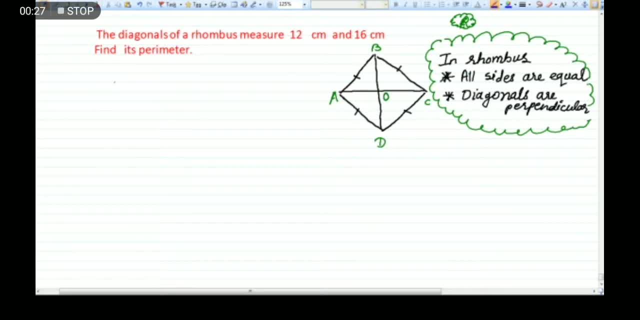 here. properties of rhombus is that all sides are equal and diagonals are perpendicular each other. so let assume that this is a diagonals. let ABC be. be the diagonal means be the given given rhombus. okay, so I write here: let the ABC be the given rhombus. now, next, where BD is equal to 12, 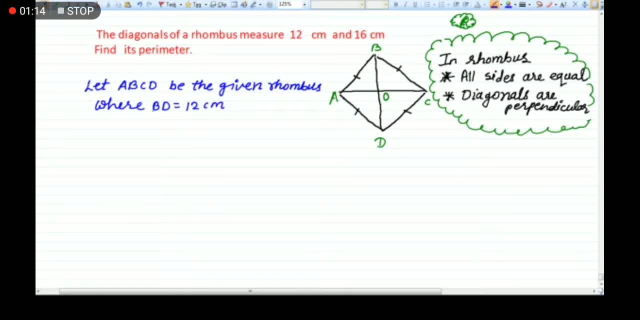 centimeter. BD is diagonal and AC is also diagonal. that how much assume that LC is a diagonal, another diagonal: that is 16 centimeter now. so look at here: BD is 12 centimeter and AC is 16 centimeter. we know from that. we know that. we know that here in rhombus. look at here diagonals. 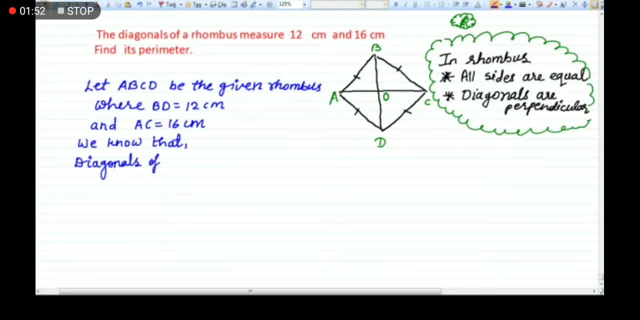 diagonals rhombus. diagonals of rhombus are bias, perpendicular to each other, you're right, basic to each other. so perpendicular to each other. yeah, perpendicular, bisect, bisect, oh, of each other. okay. so diagonals of rhombus are perpendicular by sector of each. 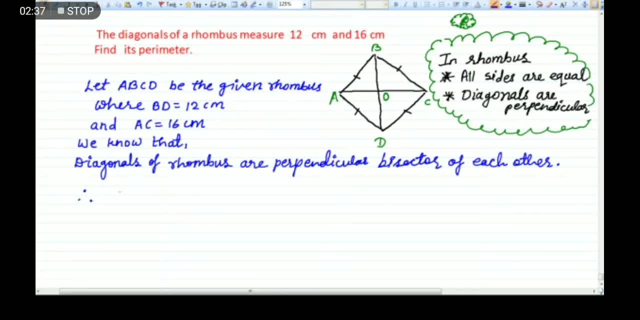 other. therefore, you see, is perpendicular to BD. so AC is a diagonal and BD is also diagonal. that is perpendicular to each other and we have to find a. o means ob. so first we have find the ob. ob is equal to bd divided by 2, because bisector means it divide two segment. this segment divide, okay, equally bd segment. 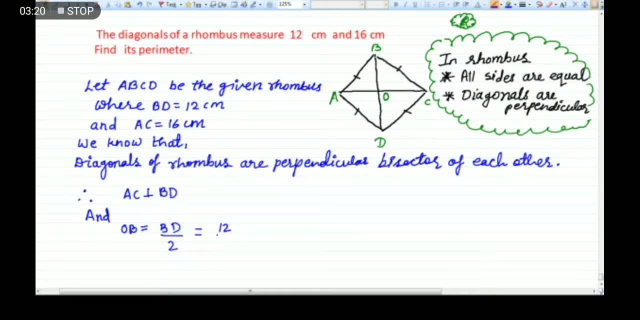 divide equally at point o, so that means bd is how much? that is 12. 12 divided by 2, that is 6 centimeter. then i will find o a and here o a is equally. divide by ac means at point a o. so 16 divided by 2, that is 8 centimeter. okay now, ac is. divide means they are bisect means equally. 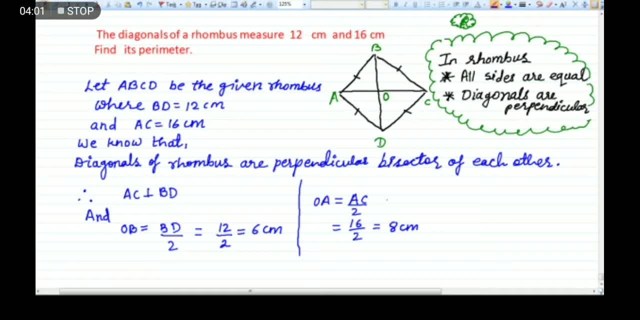 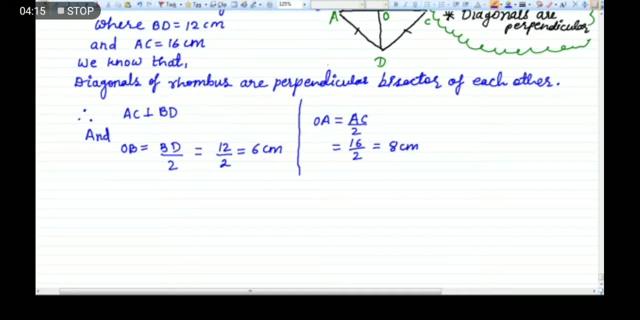 divide the ac segment into two segment, that is o a and o c. so o a, it is found here. ac divided by 2, that is 16, by 2 that is 8 centimeter. now, here see that this all are so. поэтому: Häagen realœen ada ki emdaắt. 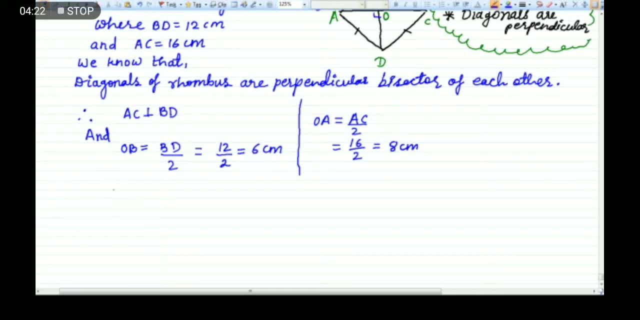 say: and these angles are perpendicular, bisect, so that make a triangle. okay. so now I'm take a triangle, a OB, a OB that is a right angle triangle so we can use. is the right angle triangle a OB at the point o, so we can use Pythagoras theorem. 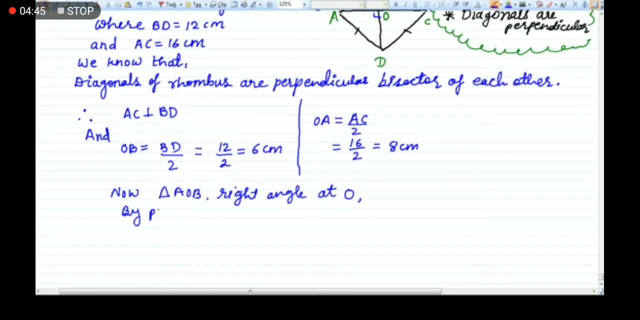 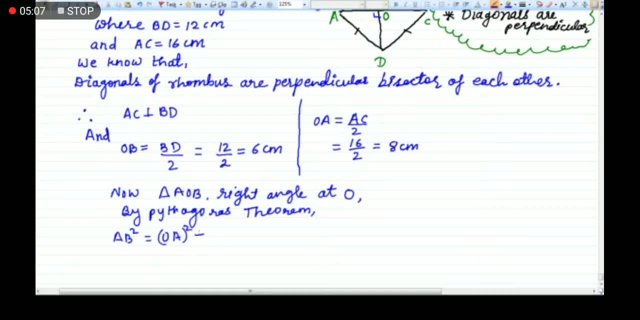 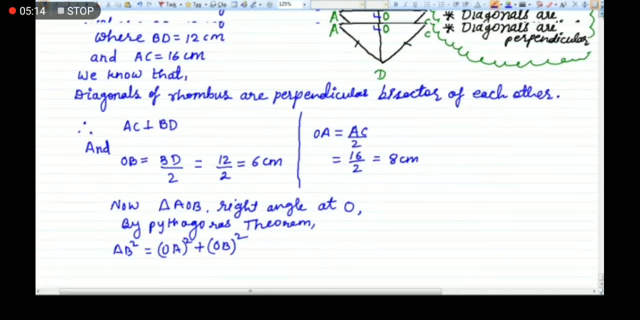 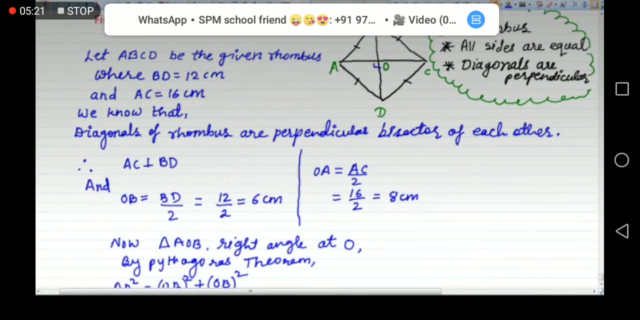 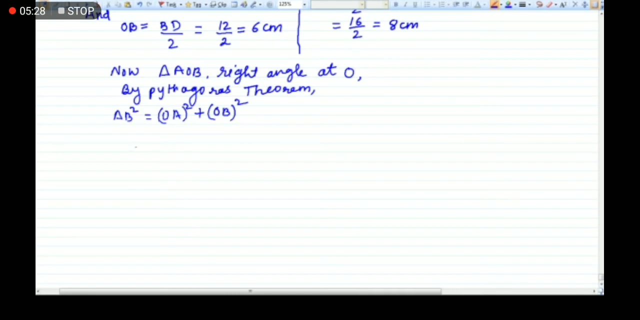 equal to OSQ plus OB square. so from this diagram you can see that. see this diagram: AB, AB square is a hypotenuse and there is a OSQ plus OB square now. so we have to find the value of that OA and OB. so what is the value of OA? that is 8, so I can write 8 here, 8 square. 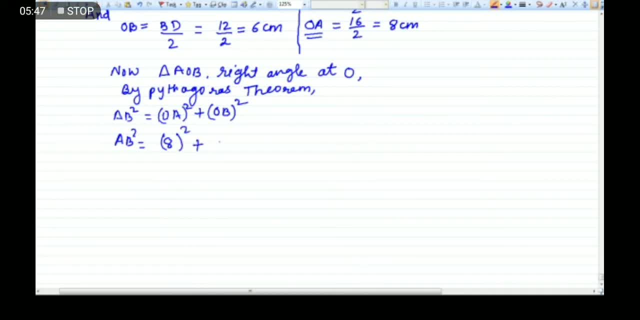 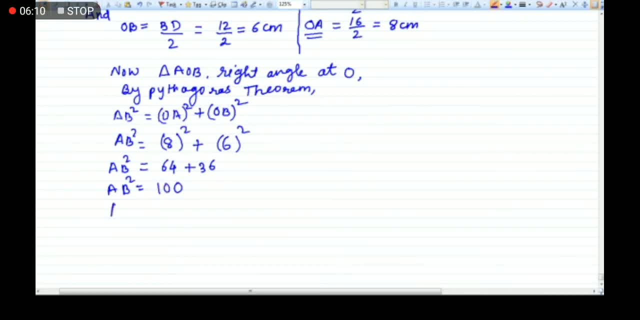 64 plus 36 is how much, that is 100. then I take square root of that number cancelling square. so square root of that number cancelling square, so we have the value of 16. so we get the value of 3 later on. this all in this bar. then, using this bar, Mr S, he writes by'd by'd. if you write by'd by'd, 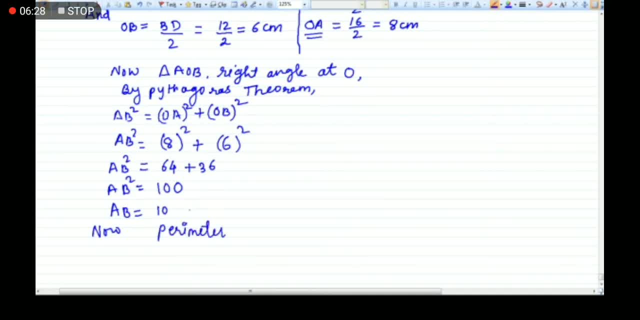 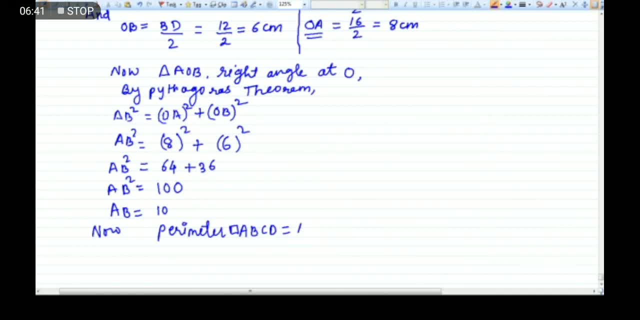 ет two nós. we'll sum this all over again. this is: we are adding instead a by V長. we are 3.65, 0.. counties changed, but a size, what are? were expanding? we are, we are. I will cheer so for jar ororenottides, though we equipped our term because we are using all of this text, which means we have to say it. 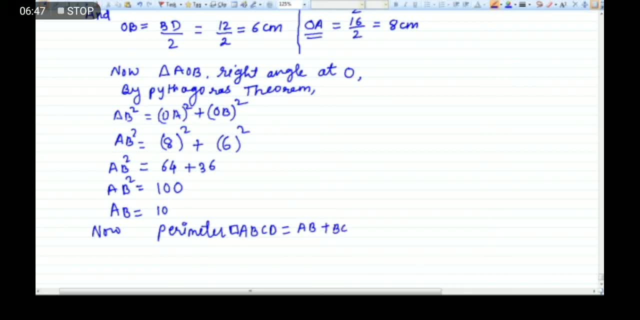 plus BC, plus CA, CD plus a D. okay, now you know from the properties all sites are equal. so I write down BC also a B, CD also a B and a D also a B. so I write to that how many a B's are there for it. because since you see that the sites of 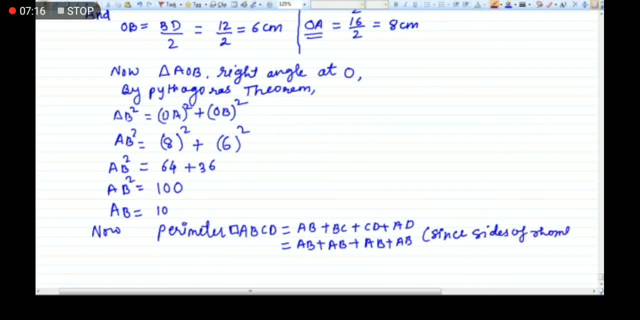 a rhombus are equal by. I'm writing a B plus a B because side of rhombus are equal. now how many be are there? that is for time maybe. so I write here 4 into a B. now I put the value of a video 4 into paint. that is 40 centimeter, so final.